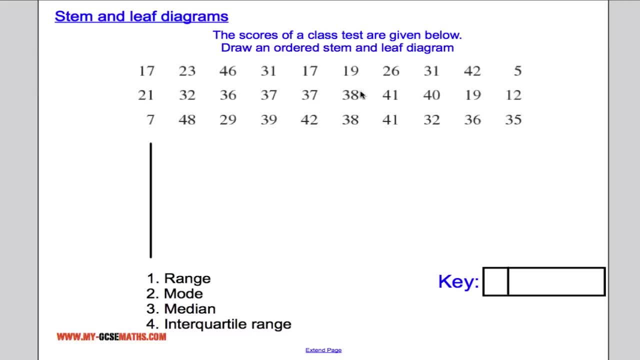 So here we have a data set and it's the scores of a class test and we're asked to arrange it in an ordered stem and leaf diagram. So it's quite a large set. So a stem and leaf diagram is a nice way to represent this data set and then use that representation to answer these questions below. 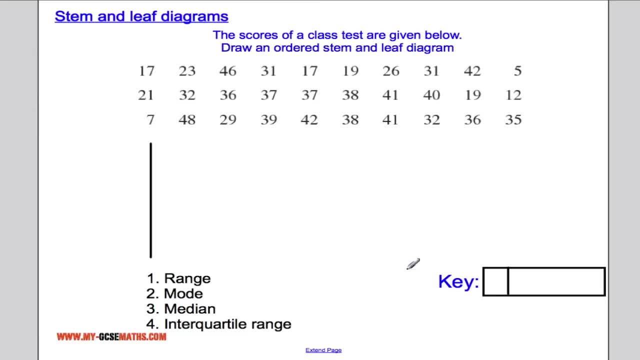 Now, the very first thing we must do is decide on a key, and that just explains how we read our stem and leaf diagram. So if I choose, for example, 21 and I say 2 with this line here, 1 means 21.. That just tells whoever views the stem and leaf diagram exactly what it means. 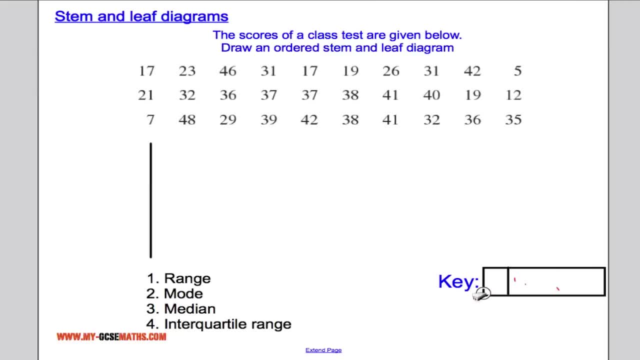 So, for example, suppose we had something like this: We had data sets using I don't know, 2.1,, 2.3, etc. I could say the 2 with the line and a 1 means 2.1. So it just explains to whoever views the stem and leaf diagram how to interpret it. 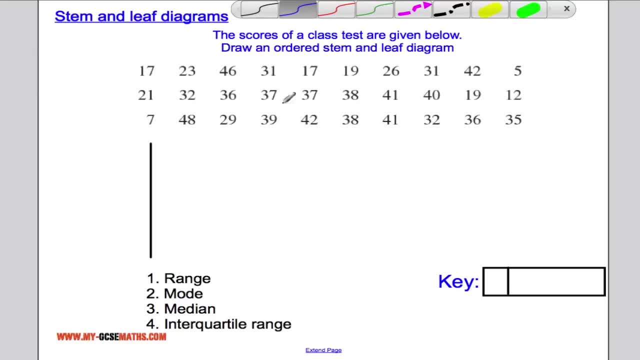 Right, So I'm going to start out by finding the smallest digit, Which in this case is 5, and I'm going to put that in my stem and leaf diagram. Now, I'm going to put a 0 here and a 5 here Because, according to our key, 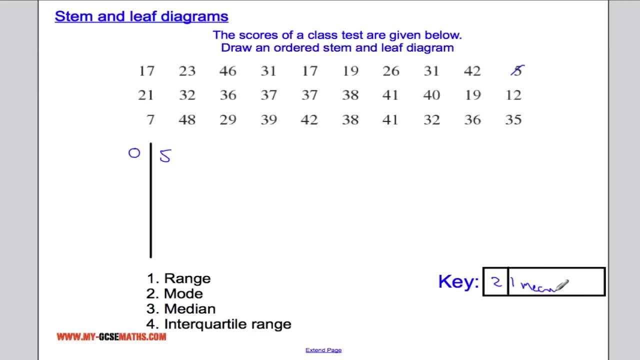 whatever is to the left of the line is the tens And whatever is to the right are the units. So we've got 0 tens and 5 units. I'm going to add in the 7.. So I just add a 7 here. Again, that means 0, 7.. 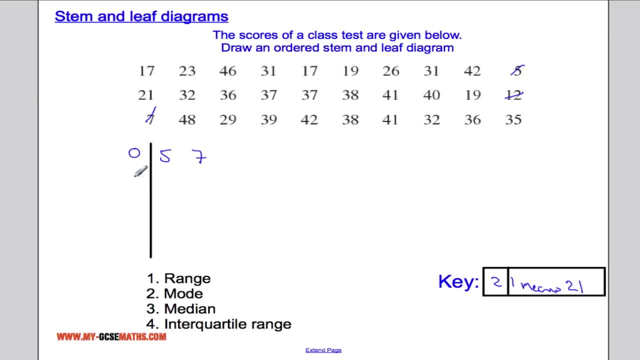 Moving swiftly along. we've got 12.. So I'm going to put a 1 here and a 2 here. Next smallest is 17.. Crossing that off. Add a 7 here. We've got 17 again. Put another 7 here. 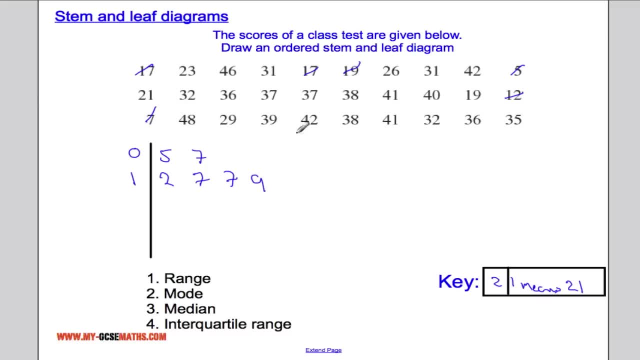 Next is 19.. So we put a 9 here, Another 19. And so on and so forth. Right the way through all the data set, Crossing them off as you go to make sure it's correct. You have all the data in your diagram and you'll end up with something like this. 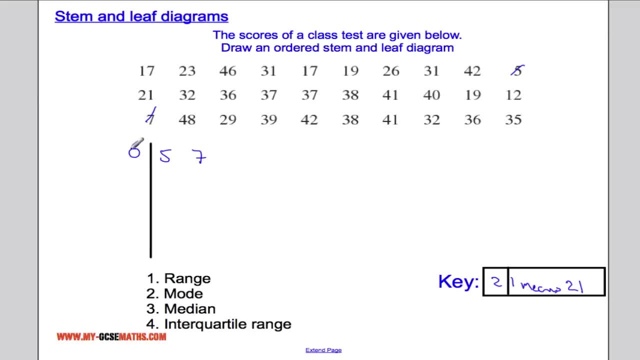 I'm going to add in the 7.. So I just add a 7 here. Again, that means 0, 7.. Moving swiftly along, we've got 12.. So I'm going to put a 1 here and a 2 here. 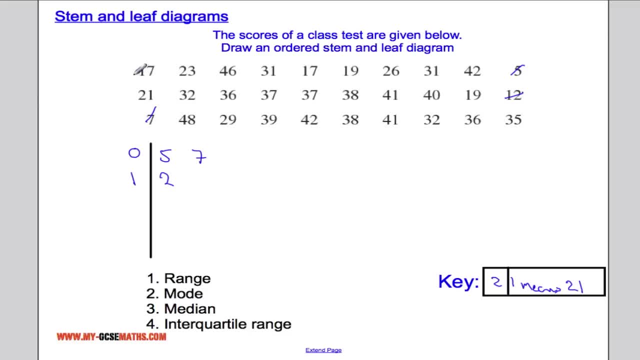 Next smallest is 17.. Crossing that off, add a 7. here We got 17 again. Put another 7 here. Next is 19,. so we put a 9. here, Another 19.. And so on and so forth. 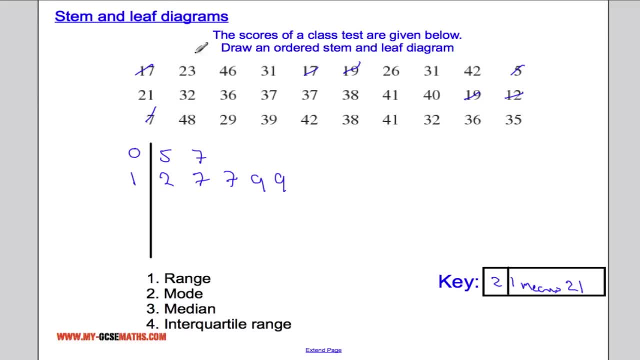 Right the way through all the dataset, Crossing them off as you go to make sure that you have all the data in your diagram, and you'll end up with something like this. So here's our stem and leaf diagram. Everything to the left of this line. here is the stem. 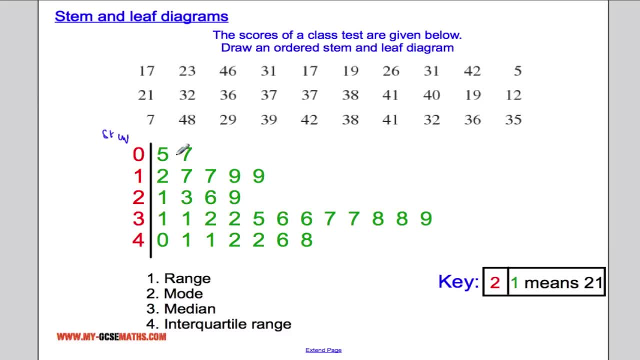 and over here, these green numbers are our leaves. Right now we want to use our stem and leaf diagram to answer these questions. So I want to work out what the range is and if you've looked at my previous video, the range is the biggest value. take away the smallest value. 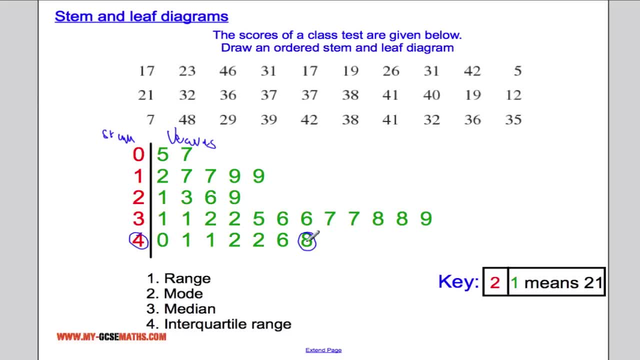 Make sure that we interpret our stem and leaf diagram correctly. so it will be 48, take away 5.. 48, take away 5, leaves us with 43.. The mode is the most common data point in our set and if we have a quick scan through our data set, 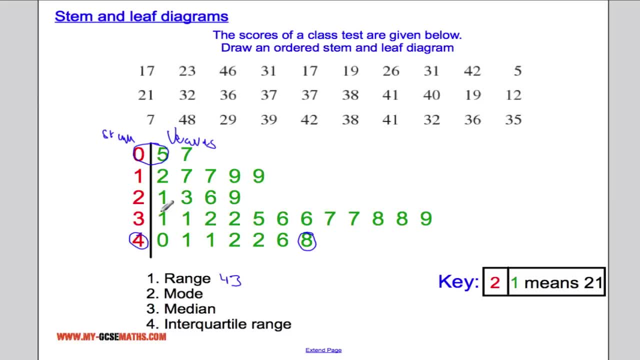 I can see that there is nothing but no mode, and we've got a couple of data points that appear twice: 31 appears twice 32,, 36,, 37,, 38, but nothing actually appears more than anything else. so I'm going to say there's no mode. 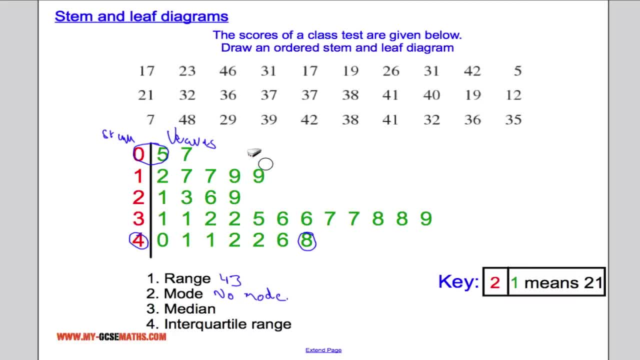 The median is found. just like we would with a list of data, I want the middle data point and again, if you've looked at my previous video, what I like to do is count all the data points. I've got 30 data points. that means the middle one. 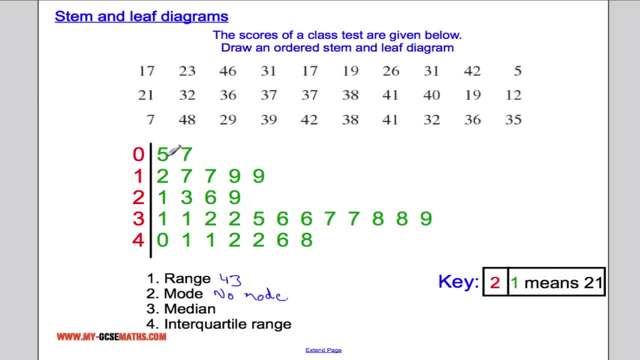 will be between the 15th and 16th data points, so let's count along one, two, three, four, five, six, seven, eight, nine, 10,, 11,, 12,, 13,, 14,, 15, and 16.. 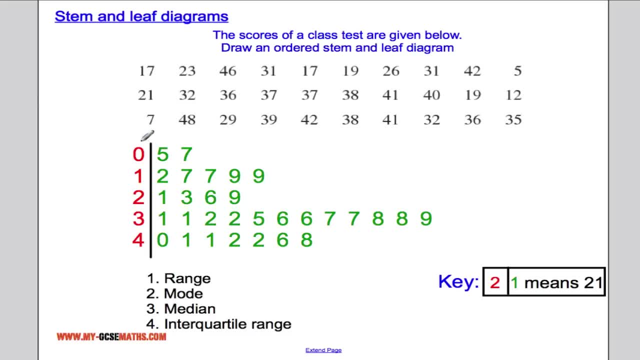 So here's our stem and leaf diagram. Everything to the left of this line here is the stem And over here these green numbers are our leaves. Right Now we want to use our stem and leaf diagram to answer these questions. So I want to work out what the range is And if you've looked at my previous video, the range is the biggest value. Take away the smallest value. 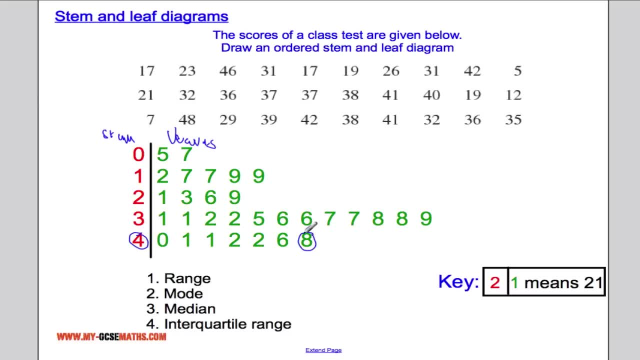 Make sure that we interpret our stem and leaf diagram correctly. So it will be 48.. Take away 5.. 48. Take away 5. Leaves us with 43.. The mode is the most common data point in our set And if we have a quick scan through our data set I can see that there is no mode. 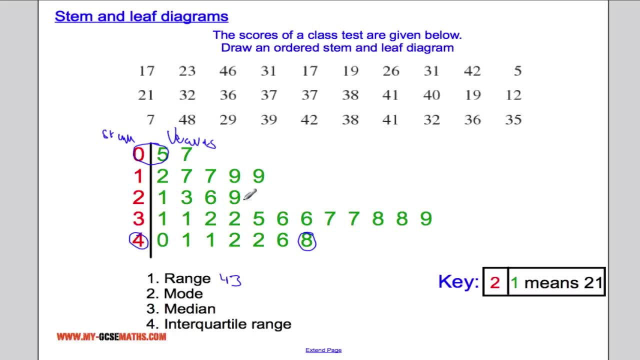 We've got a couple of data points that appear twice. 31 appears twice, 32.. 36., 37., 38., But nothing actually appears more than anything else. So I'm going to say there's no mode. The median is found just like we would with a list of data. I want the middle data point. 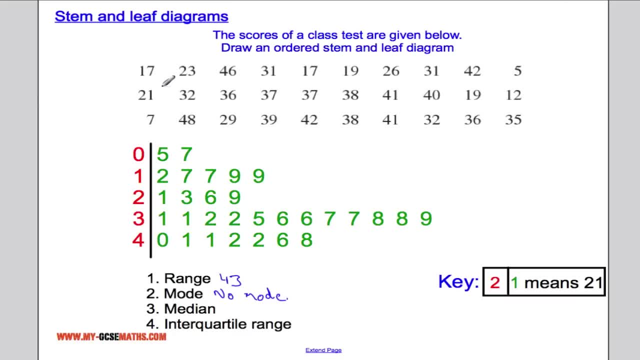 And again, if you've looked at my previous video, what I like to do is count all the data points. I've got 30 data points. That means the middle one will be between the 15th and 16th data points. 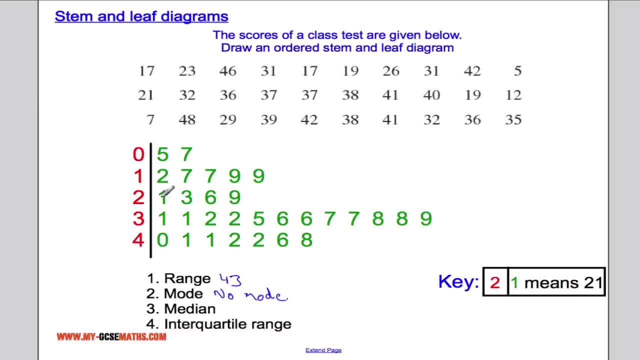 So let's count along 1,, 2,, 3,, 4,, 5,, 6,, 7,, 8,, 9,, 10,, 11,, 12,, 13,, 14,, 15 and 16.. 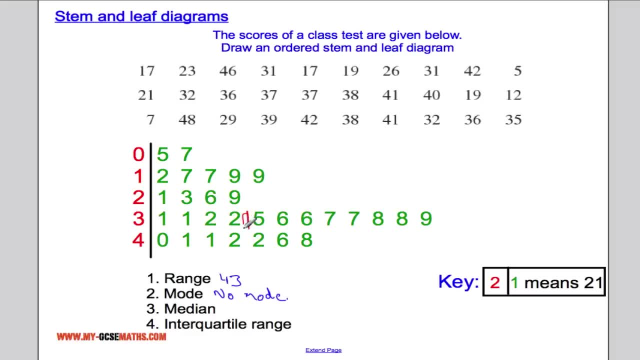 So the middle data point is in here somewhere. So what data point would be? between 32 and 35? If I add them together, Add them together 32 plus 35. That gives me 67.. If I divide 67 by 2, I get the median. 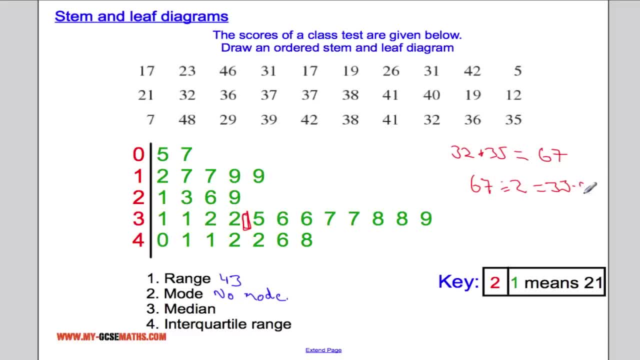 67 divided by 2 is 33.5.. So 33.5 is our median. Now I want the interquartile range. The interquartile range I've explained before is the upper quartile. Take away the lower quartile. 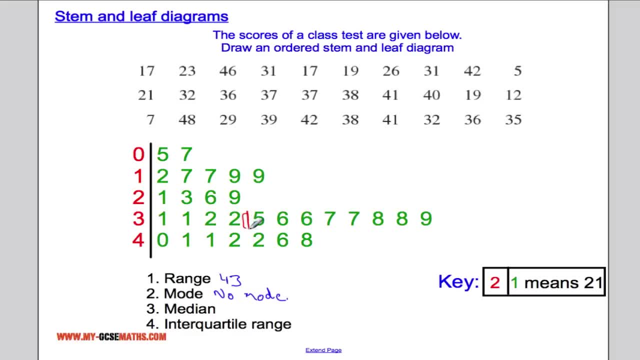 So the middle data point is in here somewhere. So what data point would be between 32 and 35?? If I add them together, 35.. 32 plus 35, that gives me 67.. If I divide 67 by two, I get the median. 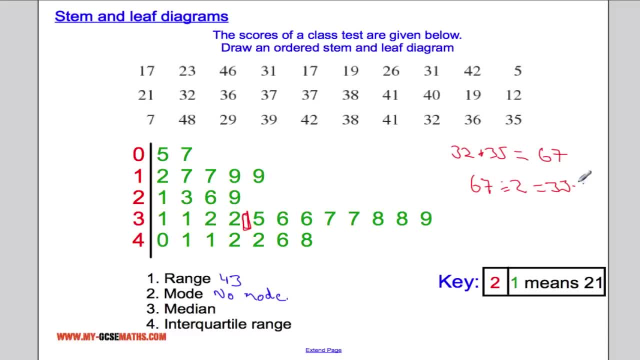 67 divided by two is 33.5.. So 33.5 is our median. Now I want the interquartile range. The interquartile range I've explained before is the upper quartile. take away the lower quartile. 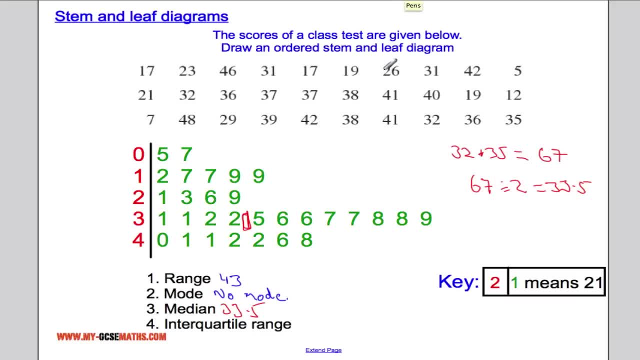 and to find the upper quartile. basically, what I want is the median of everything to the right of the median. So that was my median there. I'm gonna work out the median of this data set here, which I'll highlight for you in yellow. 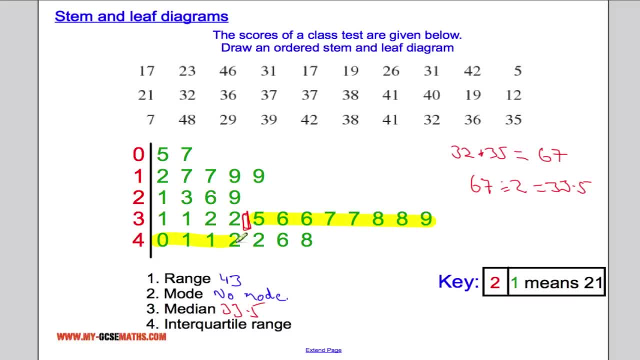 So I want the median of this data set here Right. so to the right of the median. we've got 15 data points and the middle data point of that set would be the eighth. so counting along one, two, three, four, five, six, seven, eight, 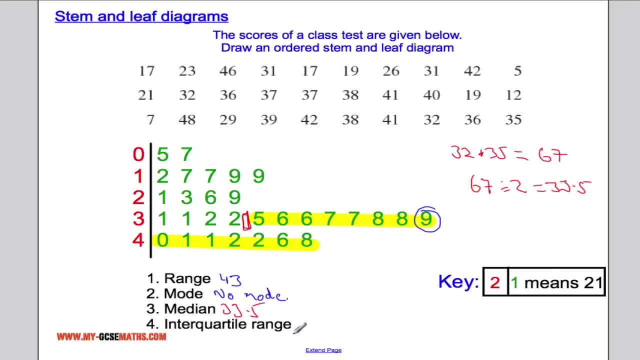 So that's the leaf, that's the stem. so the 39 is the upper quartile and I'm gonna take away the lower quartile, which will be the median of everything to the left of the median. so this part here. 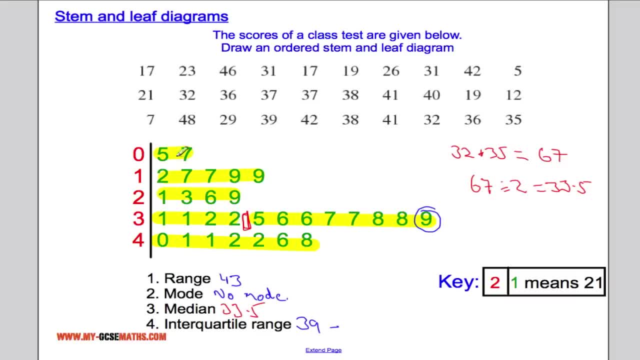 So again we have 15 data points to the left of the median. so if I count eight along, one, two, three, four, five, six, seven, eight. so 21 is the interquartile range, 39. take away 21 is 18,. 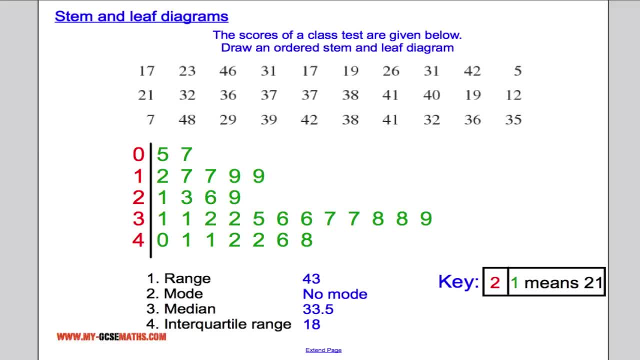 and just confirming our answers there. Another thing that's maybe worth noting is the stem and leaf diagram actually allows us to visualize the shape of the distribution really nicely. so if you actually take away the lower quartile, take away the middle quartile, take away the upper quartile, 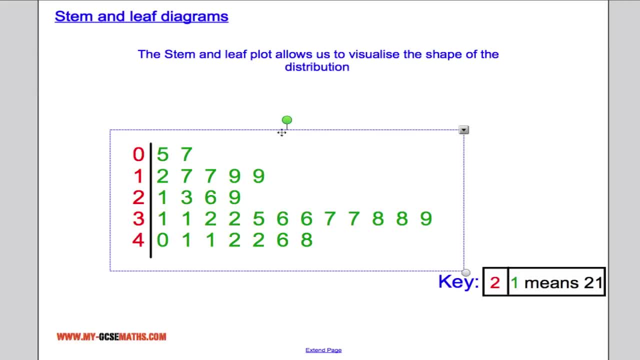 you're 0.025, so I'm gonna take away the middle quartile. take a look at this distribution. I'm gonna, I'm gonna spin it around and we can see the kind of the shape of what it looks like. let's make it a little bit. 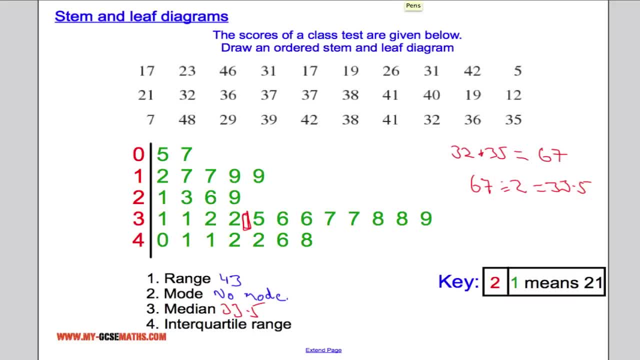 And to find the upper quartile. basically, what I want is the median of everything, to the right of the median. So that was my median there. I'm going to work out the median of this data set here, which I'll highlight for you in yellow. 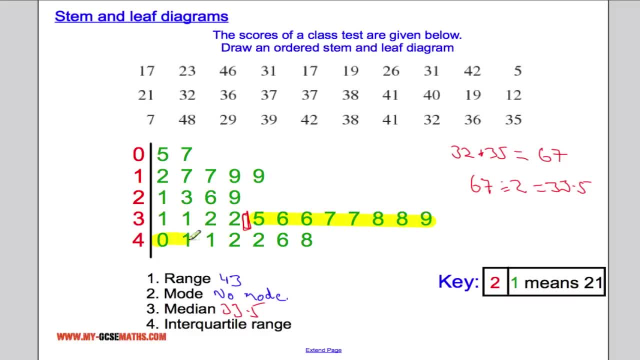 So I want the median of this data set here Right. So to the right of the median. we've got 15 data points And the middle data point of that set would be the 8th. So counting along 1,, 2,, 3,, 4,, 5,, 6,, 7,, 8.. 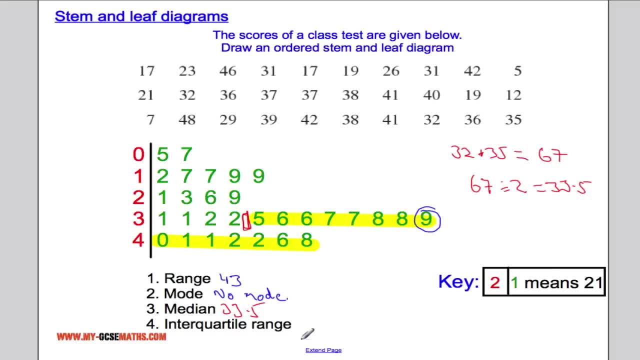 So that's the leaf, That's the stem. So the 39 is the upper quartile And I'm going to take away the lower quartile, which will be the median of everything to the left of the median. So this part here. 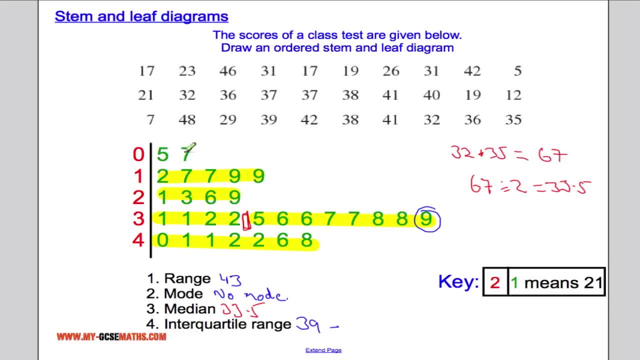 So again we have 15 data points To the left of the median. So if I count 8 along, 1,, 2,, 3,, 4,, 5,, 6,, 7,, 8.. So 21 is the interquartile range. 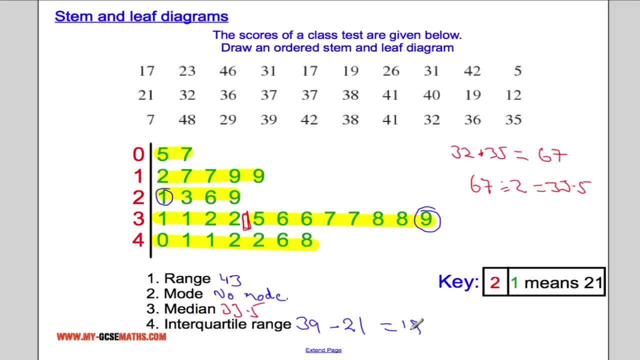 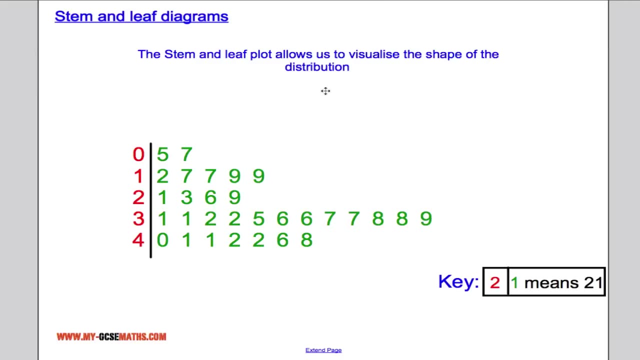 39, take away 21 is 18.. And just confirming our answers there. Another thing that's maybe worth noting is the stem and leaf diagram actually allows us to visualize the shape of the distribution really nicely. So if you actually take a look at this distribution, 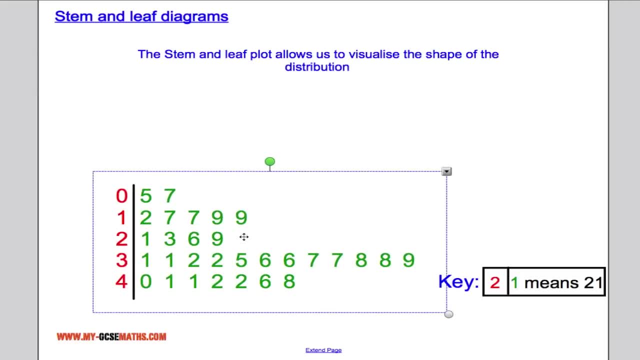 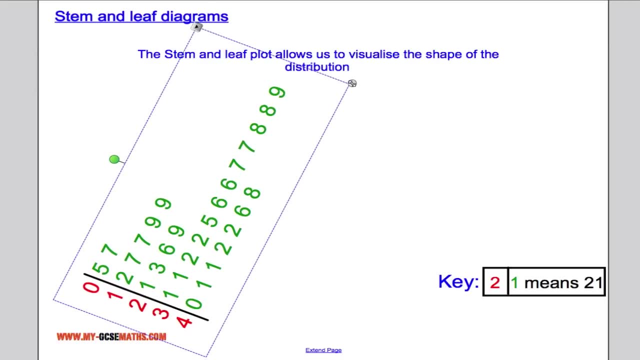 I'm going to spin it around and we can see the shape of what it looks like. Let's make it a little bit smaller So we fit it in, So we can see that the distribution has this sort of shape. Kind of tends to come up here. 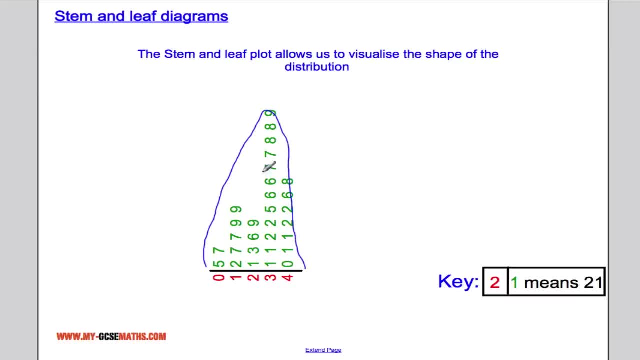 And back down, So it's actually kind of skewed to the right, And that's more or less everything you need to know about stem and leaf diagrams. So I'm going to give you a question to try. So if you pause the video and see if you can draw,